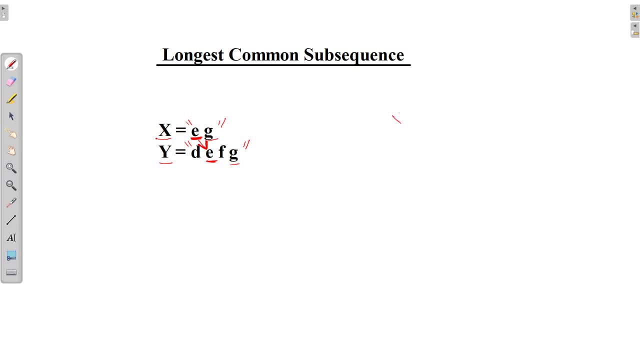 come forward to it. Let's say, if I have the example EG and in Y it is GFE, Then E is the subsequence, but G is not the subsequence because it should lie ahead of the position over here. it can be ahead or at the same. 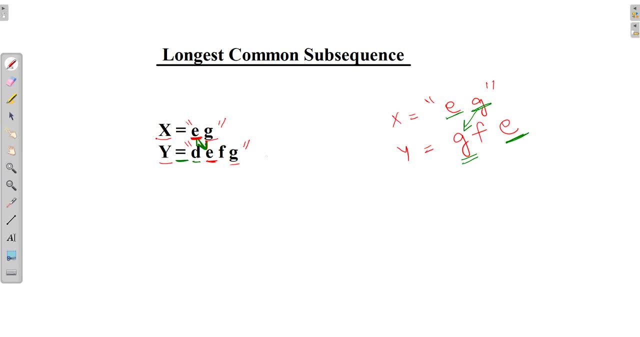 position, but not at back-position. So this point we need to keep in our mind. So let's go ahead. and firstly, we will understand this by recursion. Here we have a string X, EG, and the other string, DEFG. I have this algorithm in front of it. That has one argument in front and the other in front. So we have a strong conservativeumental and a repeating. Then we also have some other arguments which are relative, salty and effective to any individual environment as a singular property. So then I'll explain in the second video aboutanimation and then next top, final chapter, but I think I'll talk a little more about the. this is are always complex. 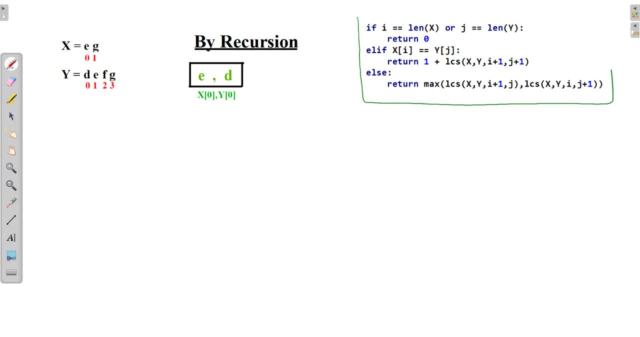 So let's go ahead. and firstly, we will understand this by recursion. Here we have a string X, EG, and the other string, DEFGaker, has a string that means this is open front algorithm in front of my screen. I'll take this- two strings and on the basis of this algorithm, 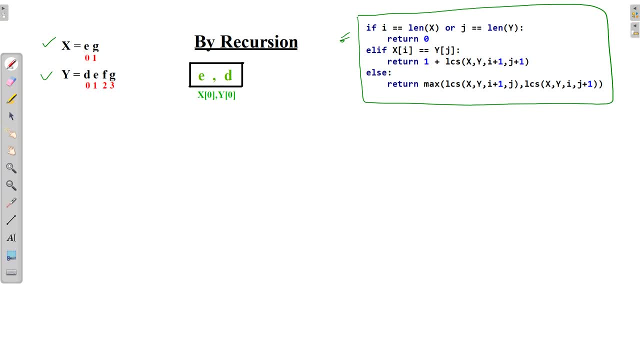 I will solve it Here. I took E and D, first letter of both string. I need to compare this E with D. is it the length of X? that is whether I is at the last point- length of X. If it is there, it should return 0. or whether E and D are equal. No, they are not, So we will go for else condition where it. 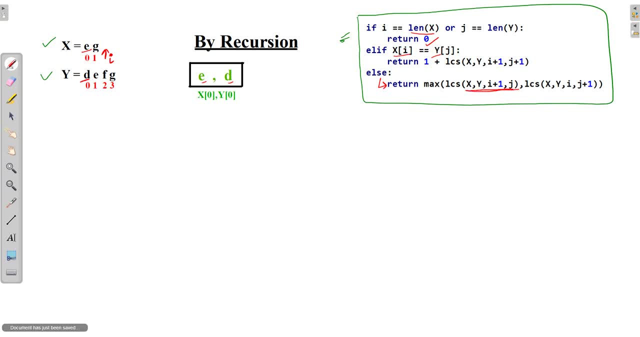 says to take firstly I plus 1 and then J plus 1, and out of these two take out the mass. So here I'll take X1, Y0.. On the other hand, I'll take X0, Y1. Here X1 is G, whereas Y0 is D. 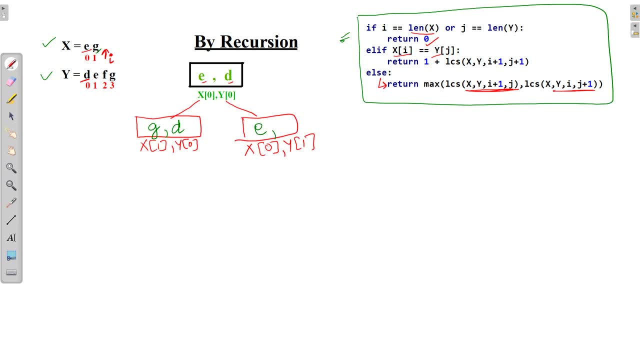 X0 is E and Y1 is E. Now we will again go ahead for GD. Firstly, I'll write all the Y's and Y's are equal, So I'll take X0, Y1.. Here X1 is G, whereas Y0 is D, X0 is E and Y1 is E. 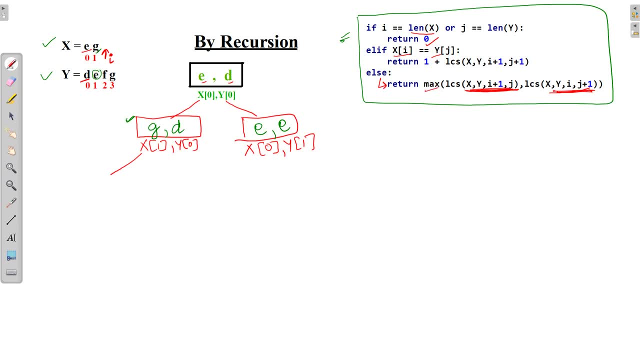 Now we will again go ahead for GD. Firstly I'll write all the Y's, and Y1 is E, Now we will all the combinations and afterwards I'll take the max of it. Now GD is neither equal, nor they are at last part of the string. So here we will again go to else part and 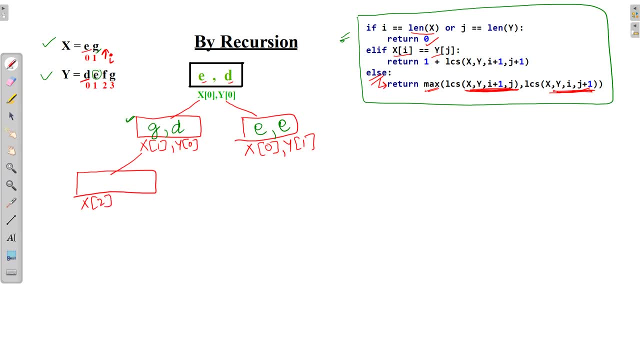 I'll take out X2 and Y0, whereas on the other hand, I'll take X1, Y1.. Now, if I see X2 is at the last point length, So I'll take X1, Y1.. Now, if I see X2 is at the last point length, So I'll take. 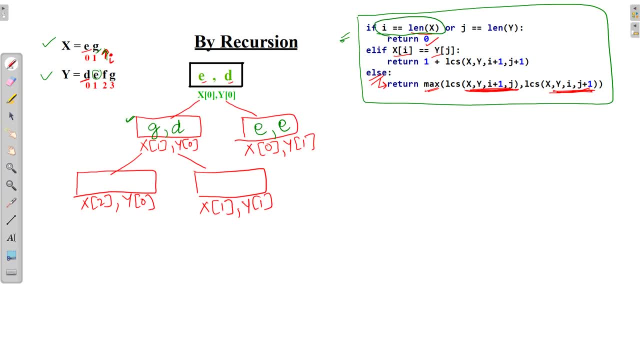 X2, Y1.. Now, if I see X2 is at the last point length, So I'll take X2, Y1.. Now, if I see X2 is at the last length, That is, it is satisfying the condition whether all the strings of X are finished. 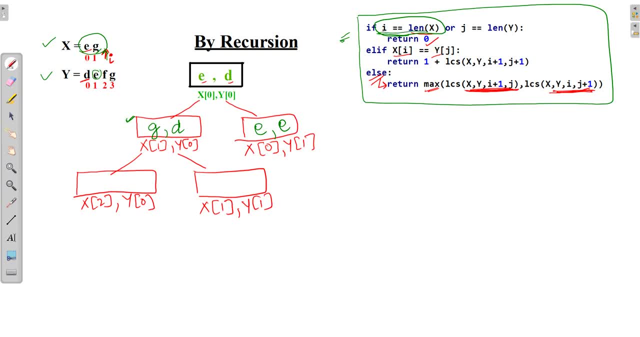 Yes, here they are finished. So here it is satisfying if condition and it says to return 0, whereas here X1 is G and Y1 is E. Now we will proceed for this. Here we will take out X2, Y1.. On the other hand, we will increment Y as Y2.. X2 is at the length of X, So again it will return. 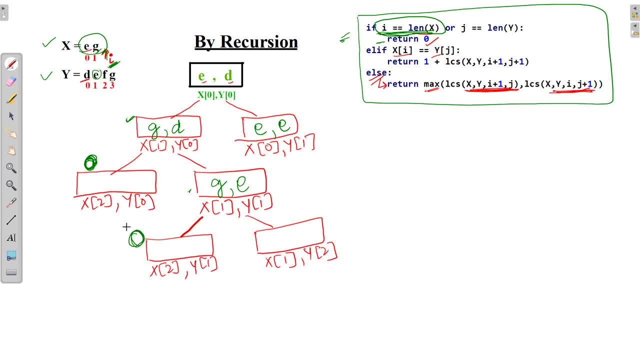 0.. So here we will get 0, whereas X1 is G and Y2 is F. So we will proceed for X1, Y2.. X1 is again for X2 and here Y2.. Whereas here X1, Y3.. X2 is returning 0. So here I'll write 0.. X1 is G and Y3 is G. 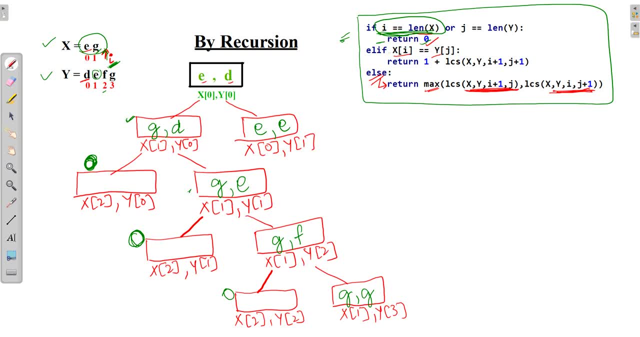 Now we can see G is equal to G. So it will go for Aleph, where it says 1 plus and the next letter of G. So it will go for Aleph where it says 1 plus and the next letter of G. So it will go for. 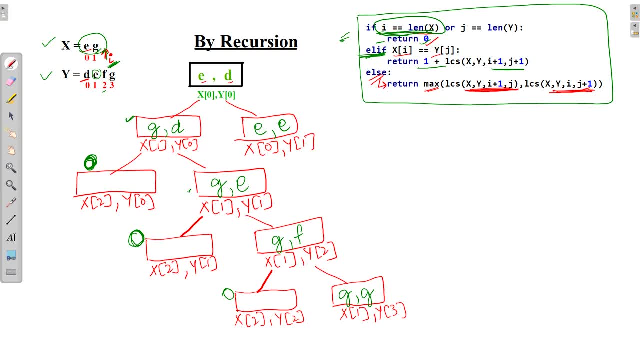 the string. So here I'll write 1 plus X2 and Y4.. X2 and Y4 are at length of X and Y, which is returning 0. So here recursion stops, and when I return here we will get 1.. Then out of 1 and 0, 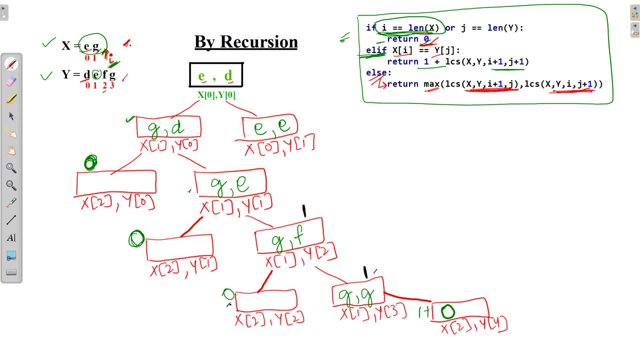 max value is 1.. So here I'll write: 1 plus X2 and Y4 are at length of X and Y, which is returning 0.. So here I'll write 1.. Then we will go to GE branch. Out of 0 and 1, max value is 1.. Then, out of 0 and 1: 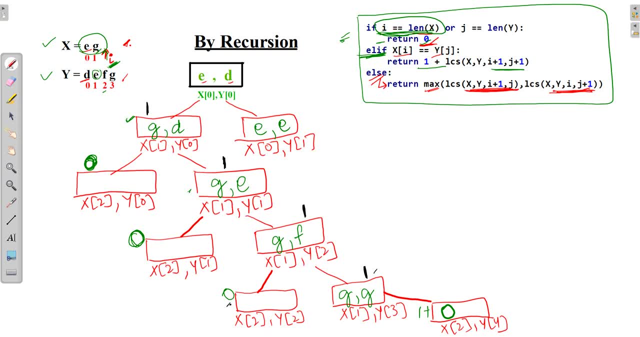 GD will get 1.. Now we are left with EE. Let's solve this, As EE are equal, So it will go for 1 plus the next letter of the string, X1.. So here we wrote 1 plus X2 and Y2.. X1 is G and Y2 is F. Now, if you look it carefully, GF, we have already solved, But still this is. as recursion. so we will solve here: X1 and Y2. G are not equal, So we will go for л part, and here we will write X2, Y2. And here X1, Y3. We will go for L and N. This recursion phenomena will be solved some length from. 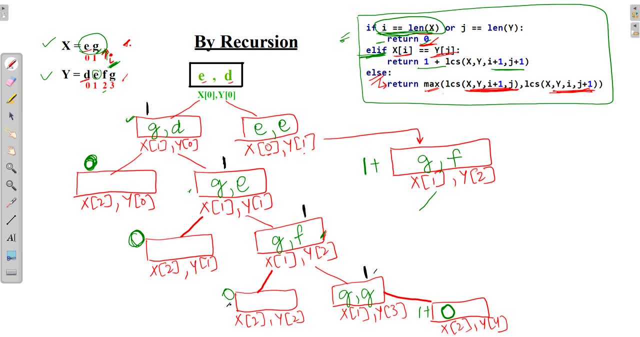 x1 and y2 gf are not equal, so we will go for else part and here we will write x2, y2 and here x1, y3. here x values ends, so it will return 0, whereas x1 is g and y3 is g. now for g. 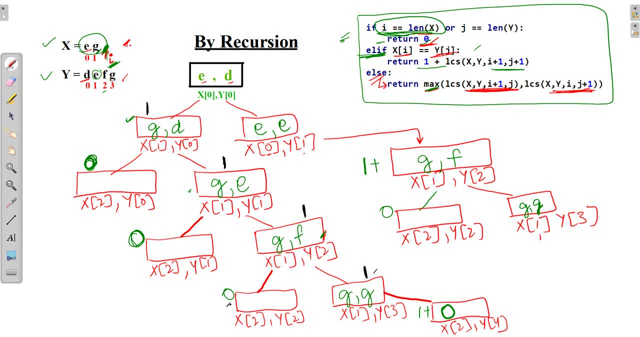 g value is equal to each other, so it will go ahead and we'll go for this return value where it returns 1, plus the next letter, x2 and y4, where we get x2. this is the last letter, same on y side, so it will go for returning 0 now. from here, value will return. 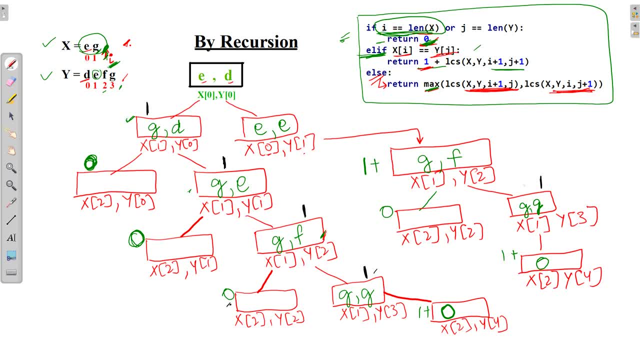 as 1- g value is equal to each other, so it will go ahead and we'll go for this return value Then out of 1 and 0, max value is 1, here 1 plus 1 is 2, so here we will get 2, out of 1 and 2,. 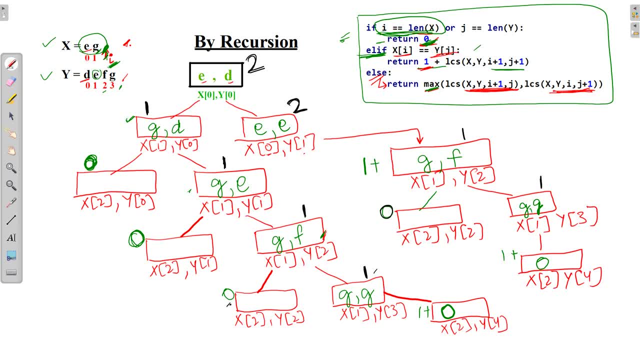 max value is 2, so here we will get 2 value as maximum. So this is how recursion works. But here you have seen that we faced a problem for G and F, as it was firstly solved here and again I have solved for its another branch. This was the small string, so it came just 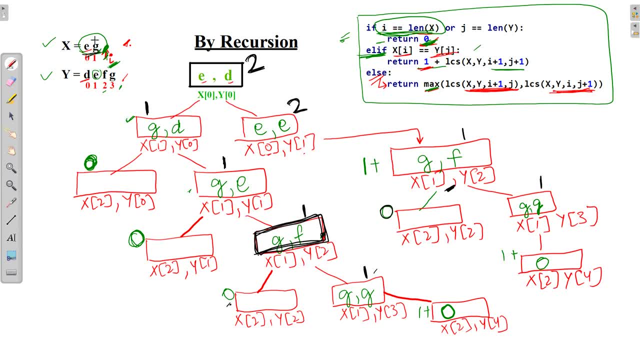 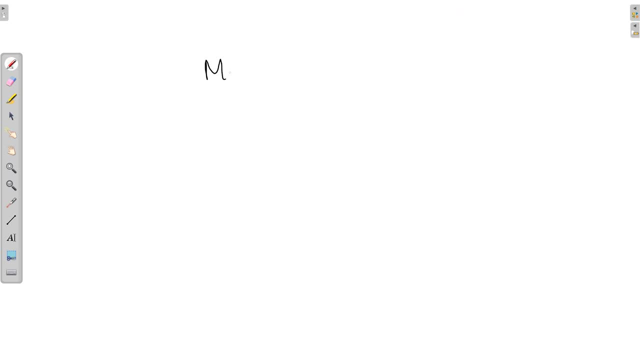 one time, But for the longest string it will have many of the branches, which is quite hectic, because if we have solved for one time, why to solve again and again? So this is where memoization comes in, Where memoization itself says to store the value. 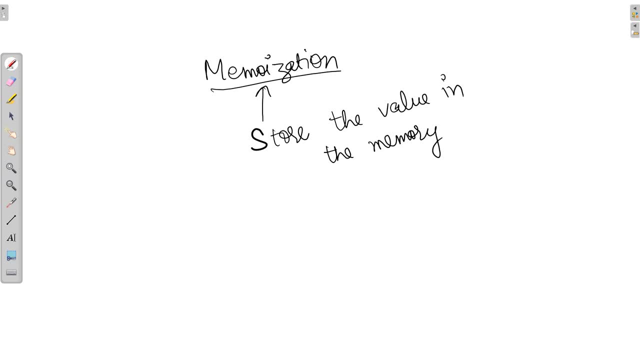 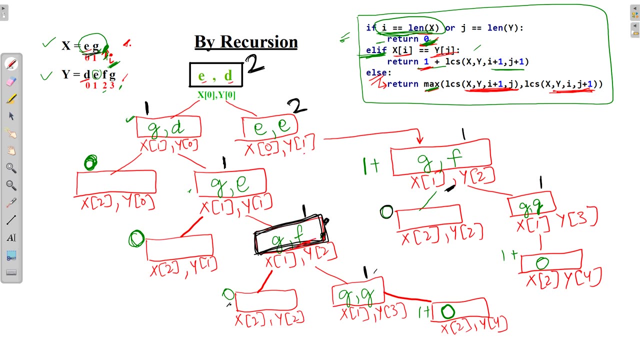 in the memory so that we can make use of this value at the next time, which we can use over here, so that if we get this GF value again, then we need not to solve for this GF. Already we have used this GF, So now we have solved for this GF. 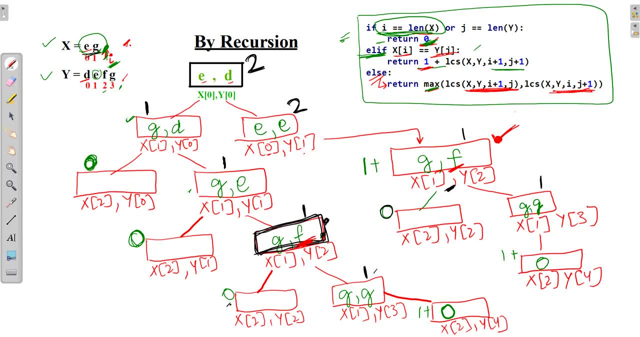 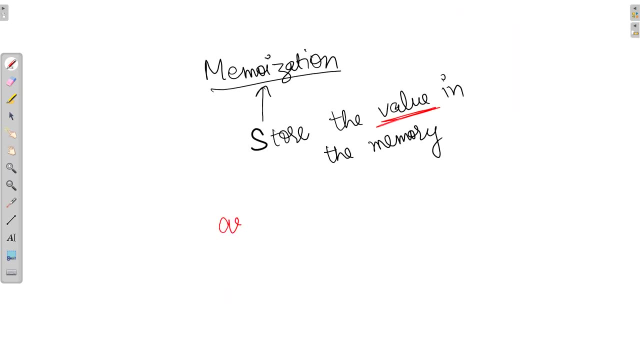 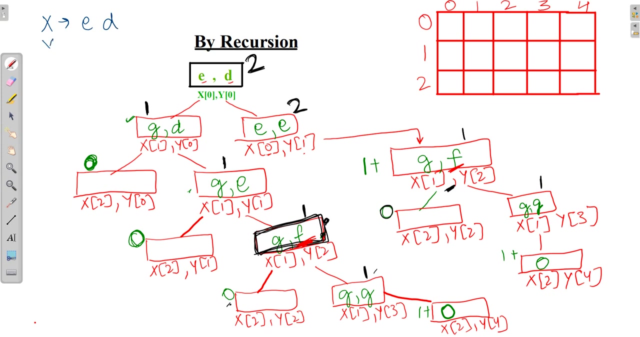 At the time of solving this. So let's see how memoization works. Recursion always works by top-down approach. Memoization also works by top-down approach. Let's see how it will work Here. we will make an array. We have the first string as ED and the second string as DEFG. 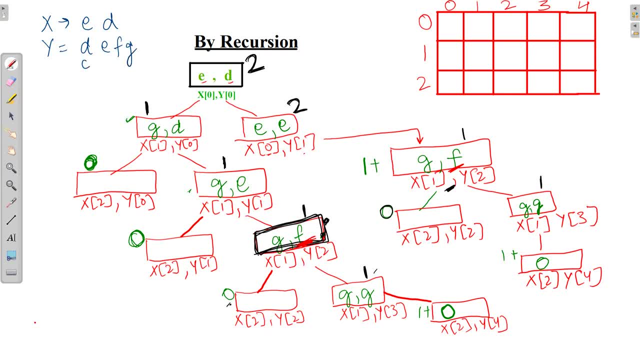 Now I have taken an array which is 0,, 1,, 2,, 3, up to 3 index, whereas 4 is for its length of Y, That is, it ends over here. Similarly for length of X as well. 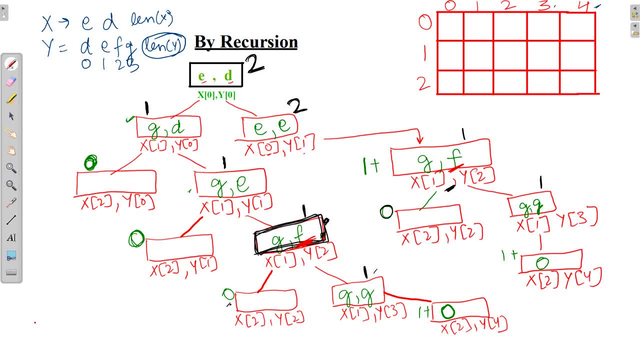 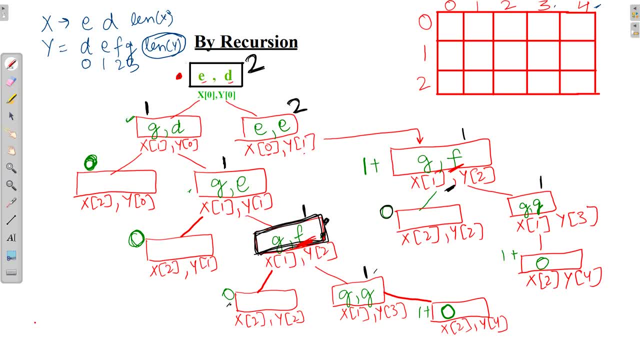 Now, when I visited the tree, when I visited last time, I will fill this array. After I visited, I will fill this array. So I will go ahead. GD for the first time. this one for the first, second and the last. 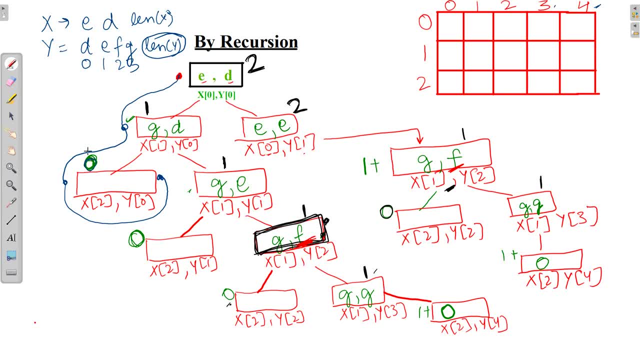 time. So 2, 0 comes first, but its value is zero, So I will fill over here, Then I will go ahead here. This is for the first time, second and this is third time, So 2, 1.. 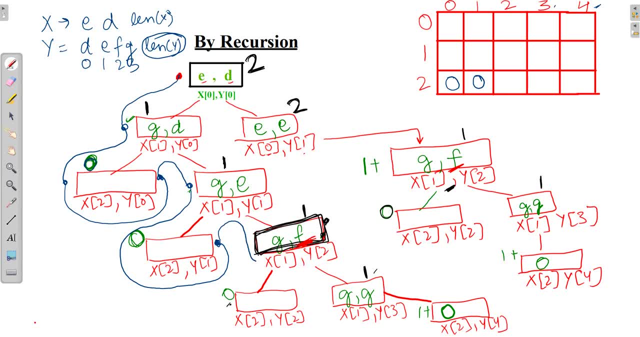 its value is 0.. Then for the 2, 2,: it's third time, So its value is 0. over here I will fill this value. Then I will go ahead for 2, 4.. 2, 4 is 0. So I will fill this value 0. Then we will. 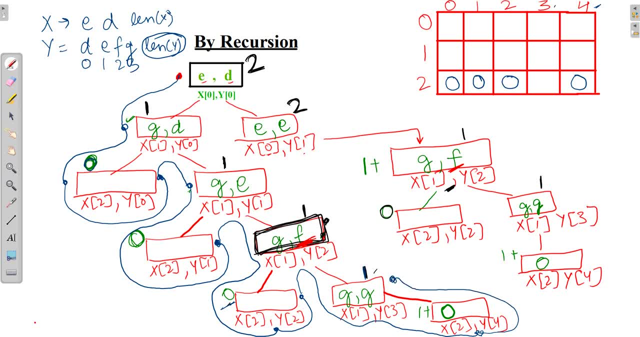 go ahead for 1, 3.. 1, 3 value is 1.. So I will write over here: 1.. Then for 1, 2, 1.. Then for 1, 1, 1.. Then for 1, 0, 1.. Then it will go ahead and it will visit 1, 2.. But you can see 1, 2 we have. 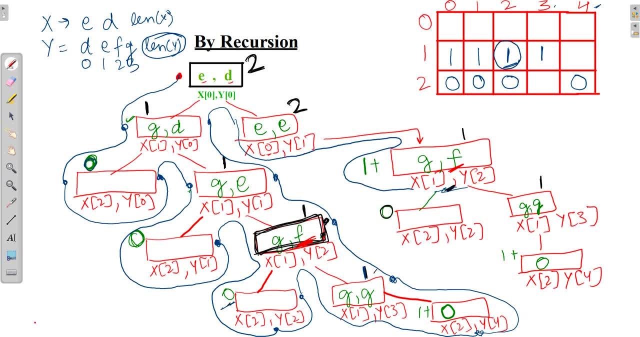 already filled over here and we need not to fill this value again. this is where memoization comes in. then for 22, it's already filled. then for 13, it's already filled. 24, it's already filled. then we will fill for 01: 01 is 2 and 002. 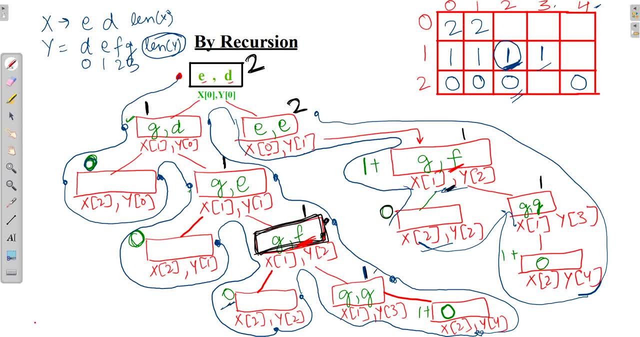 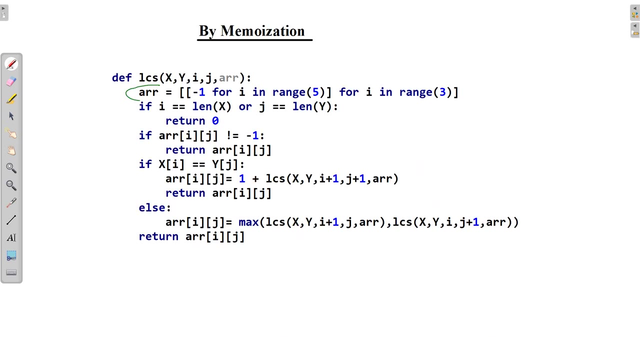 so this is how we have already stored the value in the array, which helped me while going for 12, 13 and 22. so memoization is all about storing the value so that this storage can be made use in future if we come to its coding. first, we are supposed to make an array, then the rest step. 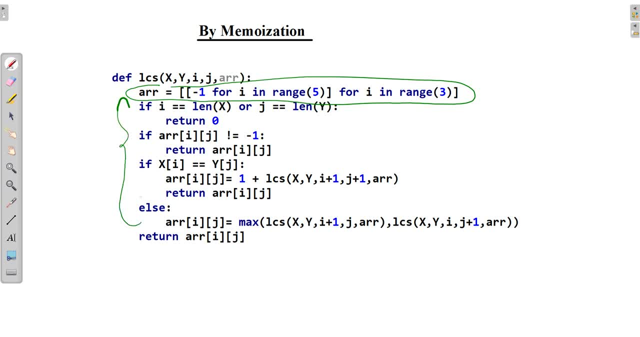 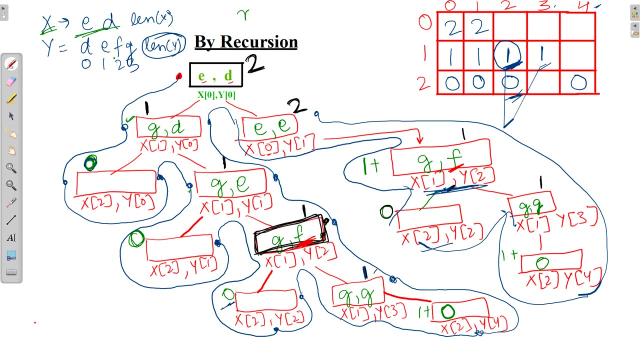 are same as recurrence. the only thing we need to introduce array and we need to fill all the values in the array. so here we have solved this problem with the help of array whose length of X, let's suppose it m, and for Y, n. so we can say m cross n, whereas if we go for recursion it's 2 to the power n, because here 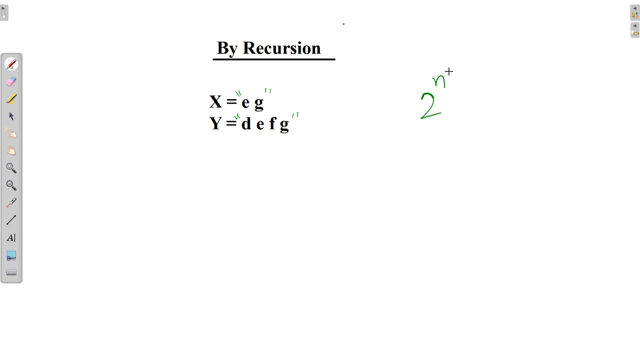 we need to solve the array of values of this array. so we have solved this problem with the help of array whose length of x, let's suppose it, m, and for y, n, so we can see m cross and whereas if we go for recursion, each and everything again and again. This memoization saves the time and solves this. 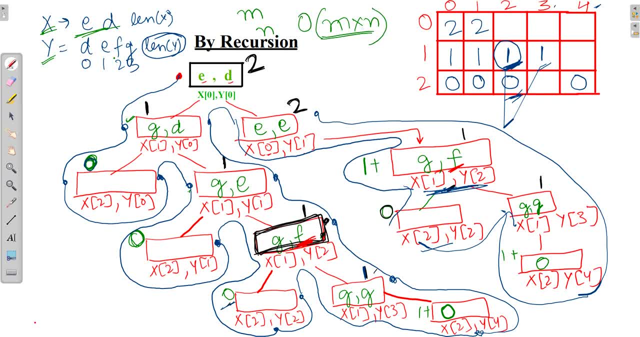 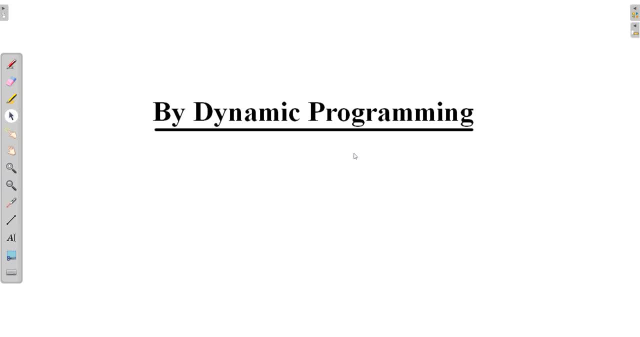 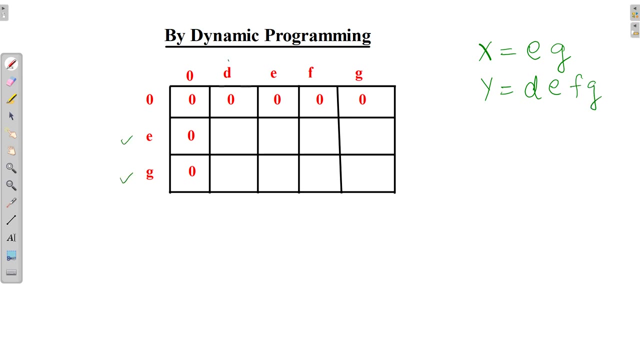 problem in order of m cross n. Now let us see this problem with the help of dynamic programming and we will solve the same problem. for x we have e g, whereas y we have d e f g. So e g I have taken over here, and d e f g, on the other hand, and with this I have taken 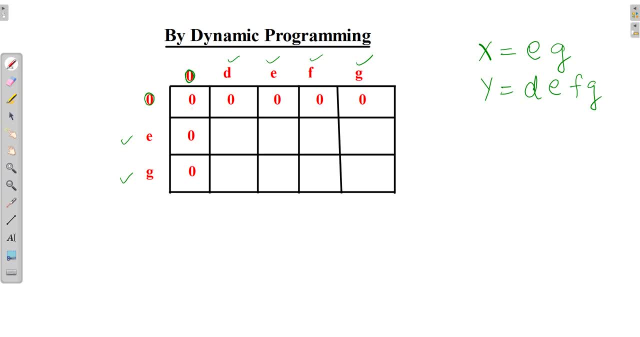 first as an empty, so that I can introduce 0: 0 on both of the x's. Now we will solve this with an algorithm where letter of one string when matches with other string, it will add 1 to diagonal and if it doesn't matches, it will go for last row and last column. 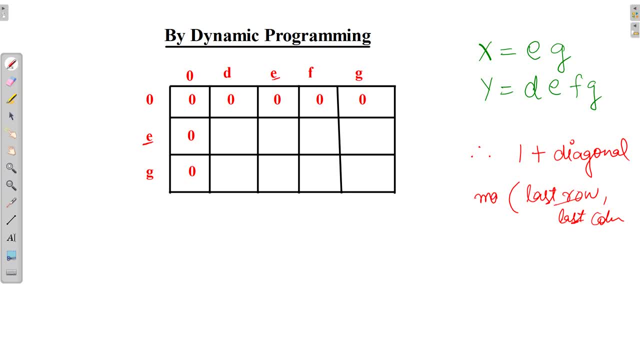 whichever value is maximum, it will store the value. So let's see it practically: where we have e, f first. e is not matching with d. that means it will go for the last row, 0 and 0. its max is 0. only so i'll write over here: 0. now e matches with e, so it will take the diagonal element, which is 0. 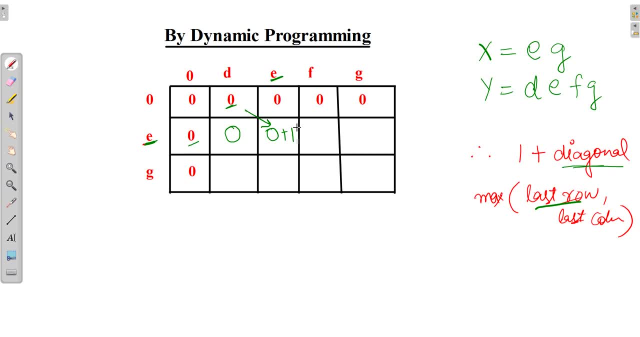 and add 1 to it, so that i'll get 1 over here now. it will check e and f. it is not matching, so it will go for 0 and 1 and will check for maximum. 1 is maximum, similarly for e and g. 1 is maximum. then for g, d: 0 and 0, g and e: 1, g and f: 1. 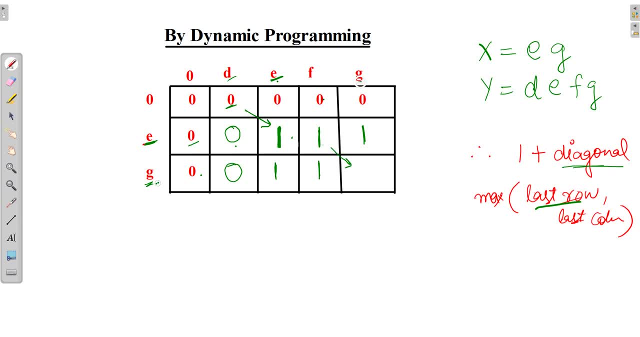 0 and 1 and add 1 to it, so that i'll get 1 over here. now it will check e and f. it is not matching. g and g are matching, so here it will take 1 plus 1 and we will get 2, so the matching value. 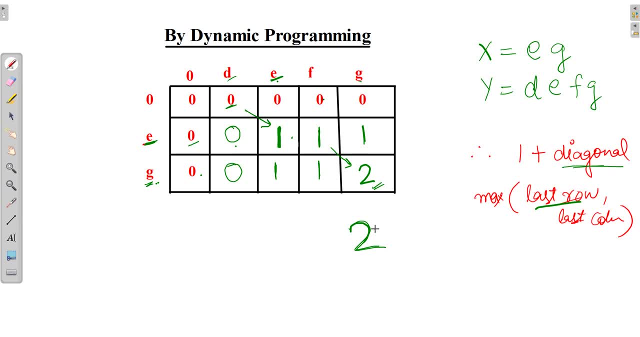 are 2 over here now, if we look for the string which are common, we will go for this arrow which is pointing over here. here it is pointing, so i will take the corresponding value g here, the arrow pointing to 1. its corresponding value is e. so e and g are the longest common subsequence. 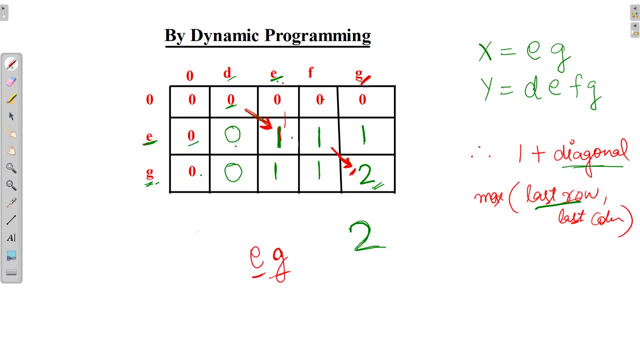 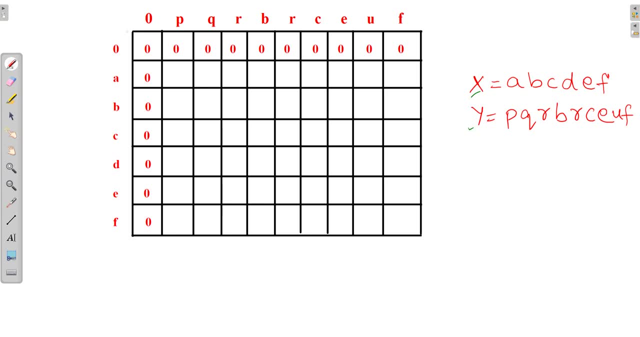 let's see this with another example. here we have two strings, x and y. i have plotted over here. now we will check this using dynamic programming with the same strategy. here we will see for it a whether a is matching with p. no, so it will look for the last row and last column: 0, 0. so 0 will be the maximum value. then a and q: 0 a, r, 0 a, b, 0 a, r 0 a, c 0 a, e, u, f, a is not there, so all values will be 0. then we will go for b. 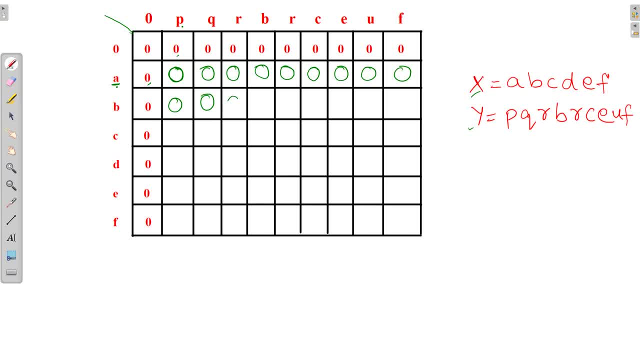 a and q: 0 a, r, 0 a. b, 0 a. r, 0 a. c, 0 a, e, u, f. a is not there, so all values will be 0. then we will go for b. Q is not matching. B is not matching with R. Now here we got B, so it will add the one value. 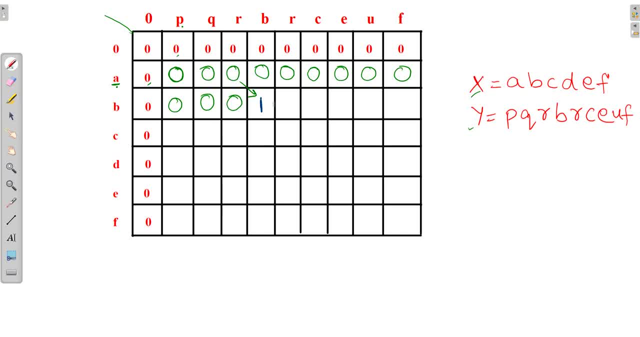 to the diagonal element, so that I will get value 1.. Now we will proceed further. B is not matching with R, so it will take the maximum value out of 1 and 0, 1, 1, 1, 1.. Then for C, C is not matching. 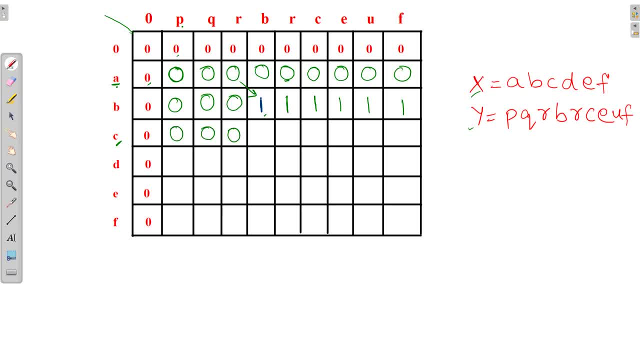 with P, Q, R. now, here we will take the maximum value 1, 1.. Now we got C matching with each other, so we will take 1 plus 1, and here we get 2, then 2, 2, 2.. Then D is not matching with P: 0, 0, 0. Neither matching with B, so we will get 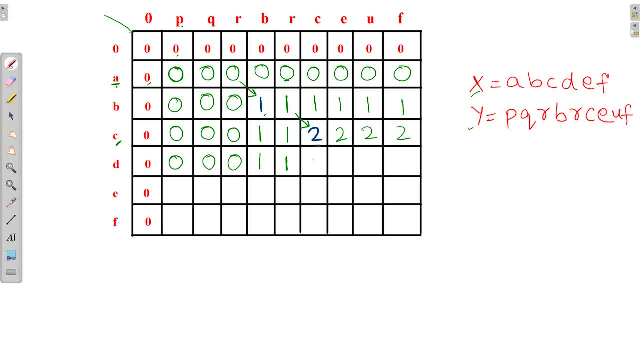 1, R, C, here 2, D is not matching with E, U, F, Then we will look for E: 0, 0, 0, 1, 1,, here we get 2.. Now, here E matches with E, so here it will point 2 plus 1, and this time we: 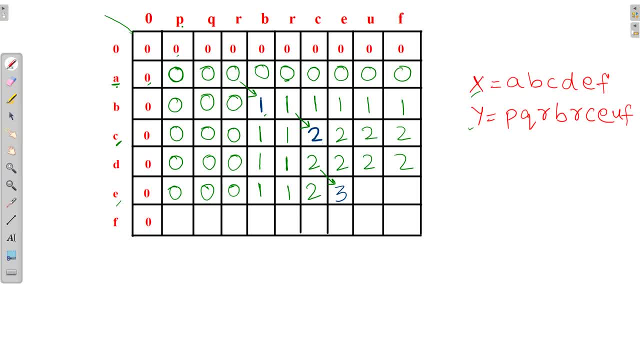 will get 3 value. Now it will check for E with U, no, no. Then for F: 0,, 0,, 0,, 1,, 1,, 2,, 3,, 3, and here F matches with F, so that we will get diagonal value and plus 1.. And we got the longest common. 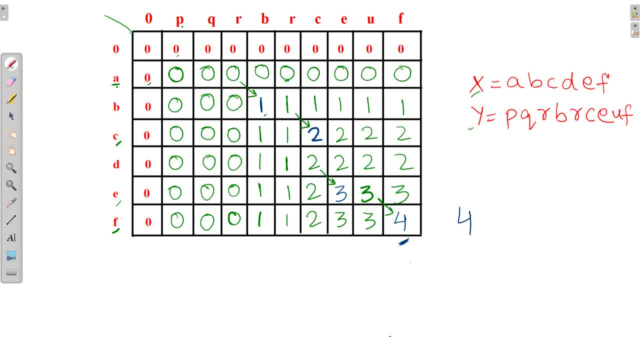 subsequence value is 1.. Now we got 2,, 2,, 2,, 3,, 3 and here F matches with F, so that we will get value as 4.. Now we check the string for common subsequence. We just need to look for this blue. 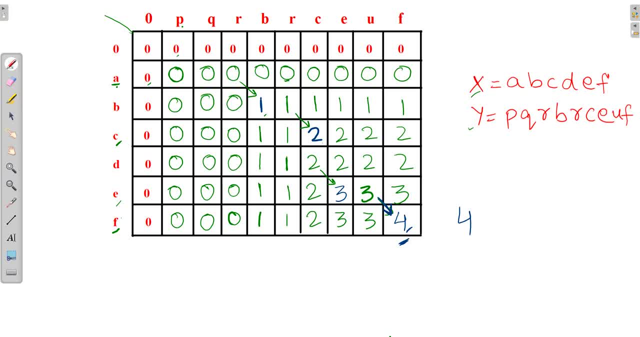 color where arrow has been pointed. 4, now we will look for its corresponding value, which is F, then this 3, which is E, now this 2, its corresponding value is C and here B. So B, C, E, F are the 4 letters of the string which makes common subsequence. 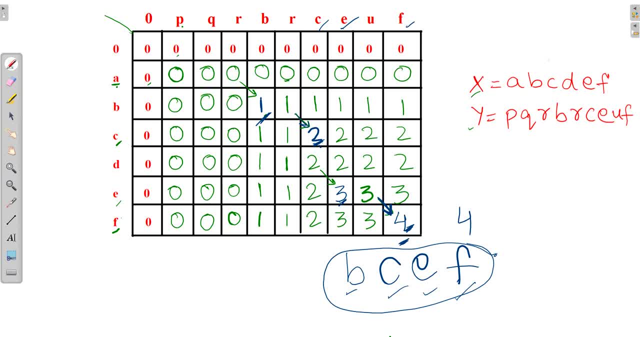 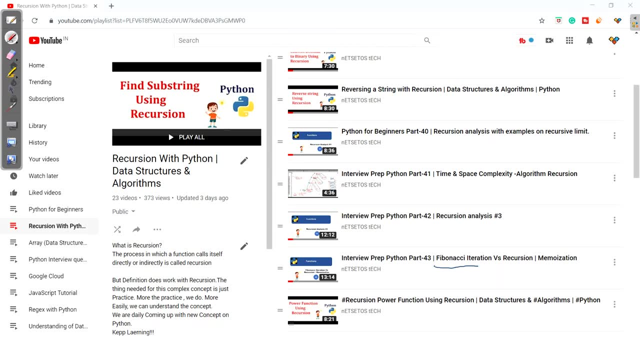 So this is all about longest common subsequence, which you can solve it by recursion, by memoization and also by dynamic programming. And if you want to practice this, I have also made Fibonacci which is by iteration, recursion and memoization, So I will recommend you to go through it Here. I 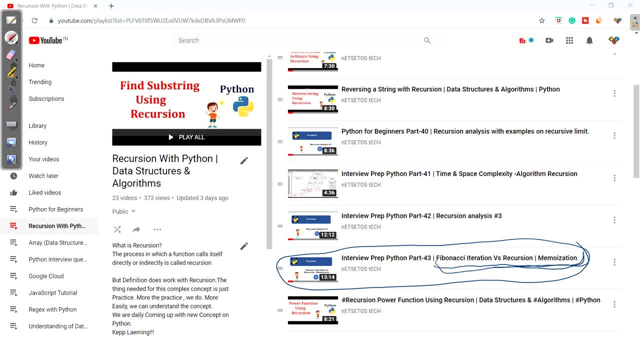 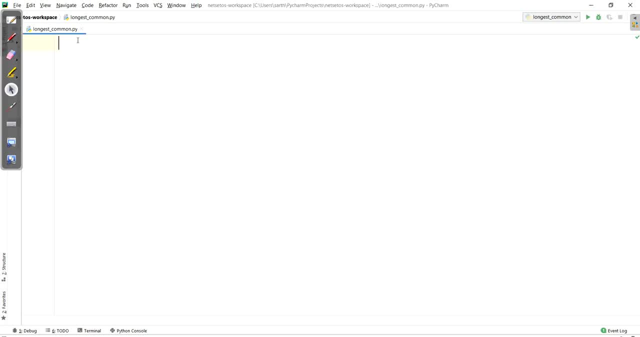 have discussed it with recursion and memoization way. So with this let's make a program on dynamic programming. Here I am on PyCharm and I have made a new file longest common. So let's start by making function def. I will take the smallest name and I am going to take the longest common, So let's. 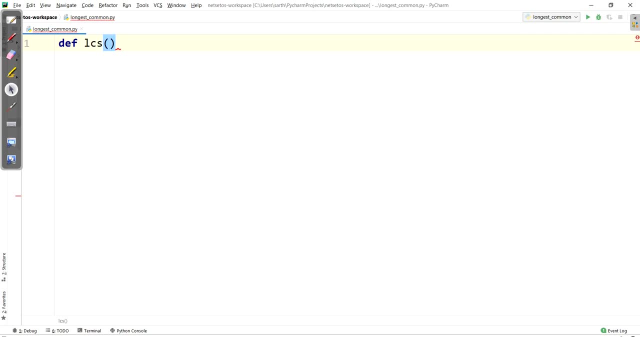 take the smallest name, LCS, and two strings, X and Y. First I need to make an array 2D array. So Python has a little bit different syntax. So first two square brackets, 0 for I in range. Let's decide. 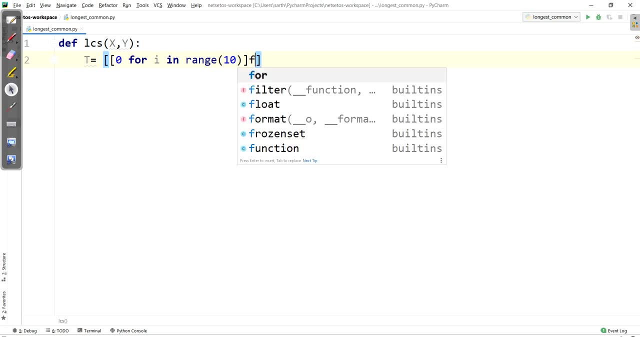 this as 10 and the other one for J in range. So I am going to take the smallest name, LCS, and two strings, X and Y. By default, I will make it as zero. Now we will define for loop for I in range. 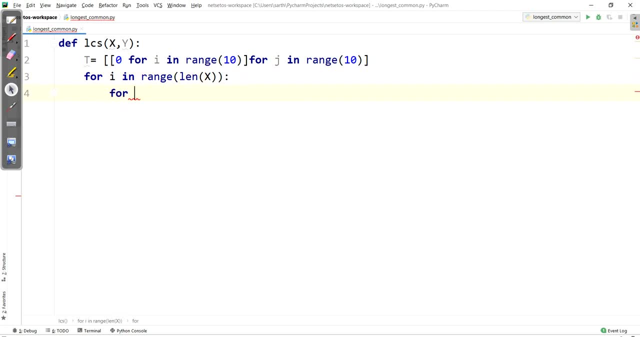 len of first string and the other loop for J in range len of Y In dynamic programming. there is one plus point: If you understood the concept, you can write its program in seconds. So here we just need to introduce two conditions.